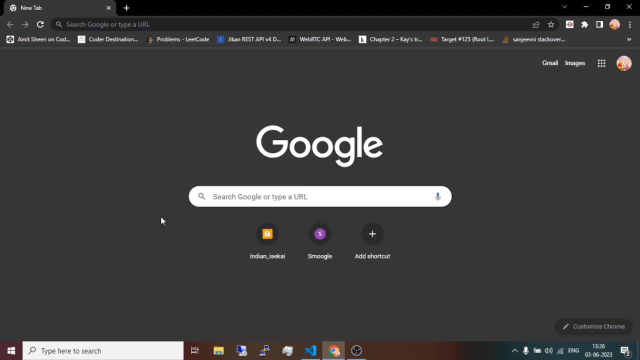 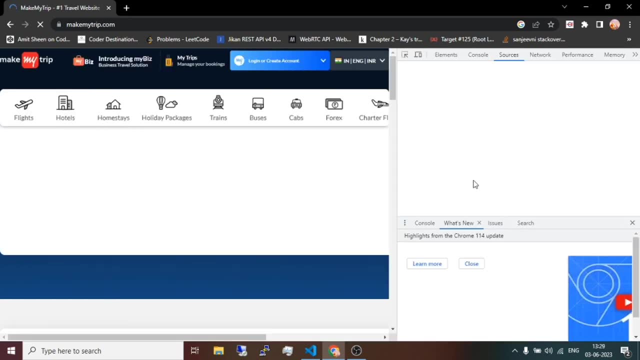 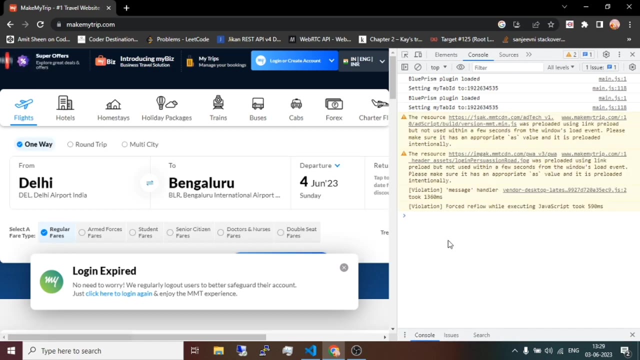 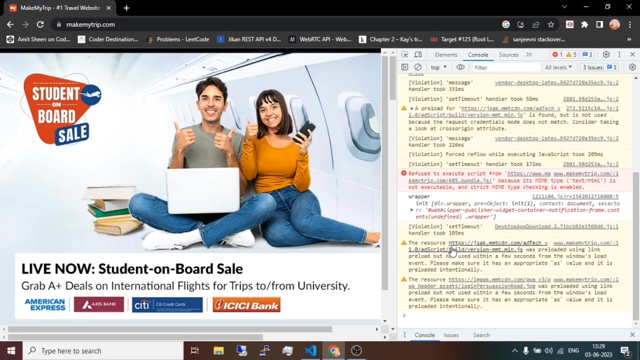 exercise. just let me visit any website randomly. so let's first get started with the documentgetElementById. so documentgetElementById is a method using which you can access any element inside your document by just passing the ID of that particular tag. so let me tell you here something. so the ID which I am going to talking about is: 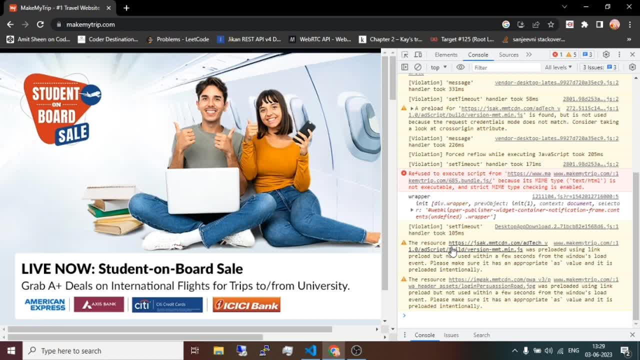 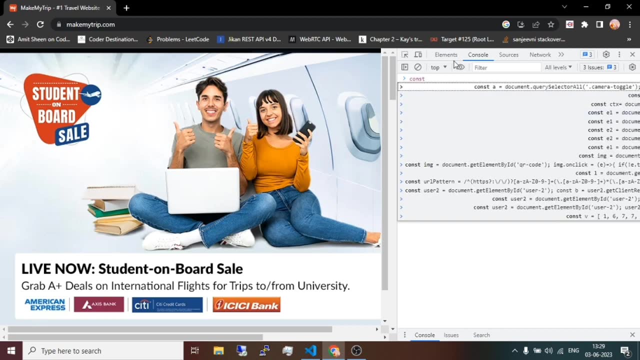 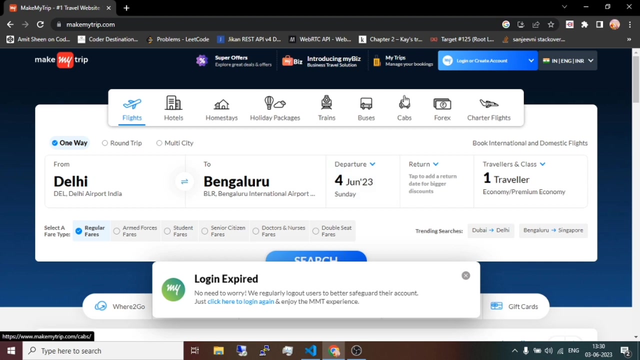 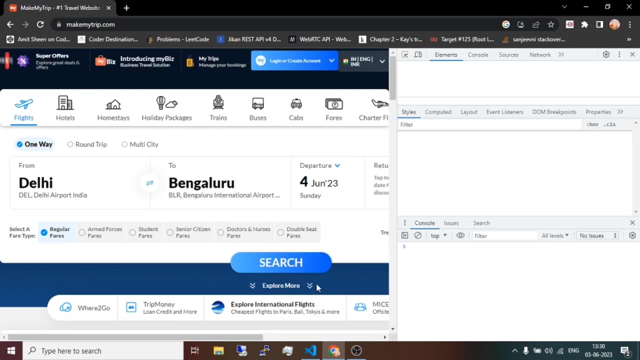 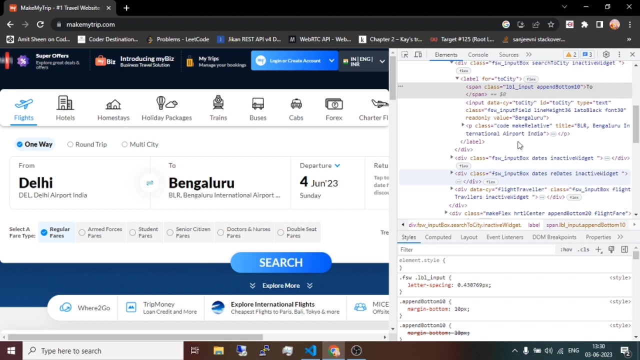 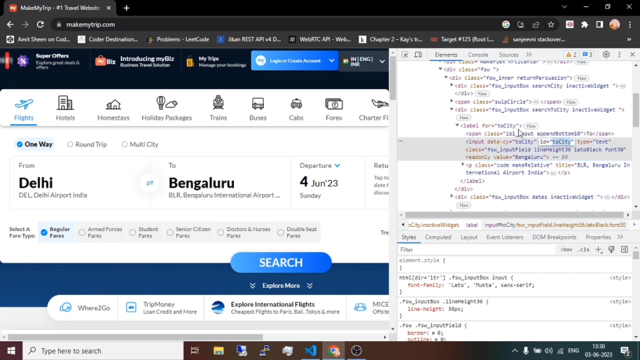 unique to every tag. so if in the overall document you can only have one unique ID attached to single tag in that overall website, let me first inspect any element which have some ID attached to it. so here we got this ID to city, so let me copy it and using our documentgetSelectedByElement. 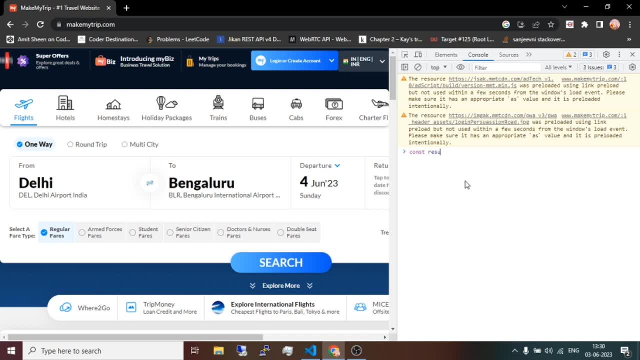 so let me store the result in this result variable, so let me print it in front of you. so we are getting that particular input tag which we have selected using the documentgetElementById. so now you can perform any different kind of a task on this particular tag. you can change. 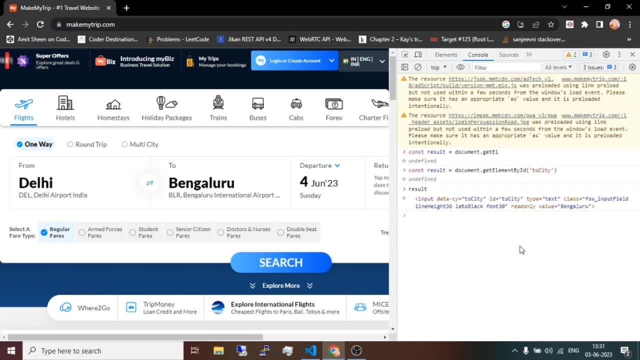 its value. you can just type another value inside it. you can change its style as well, with its size and height. anything you can perform using this particular result we are getting here. so let me show you using just by simply changing the style of this particular tag here. so let me make it its background red here. so, as you are, 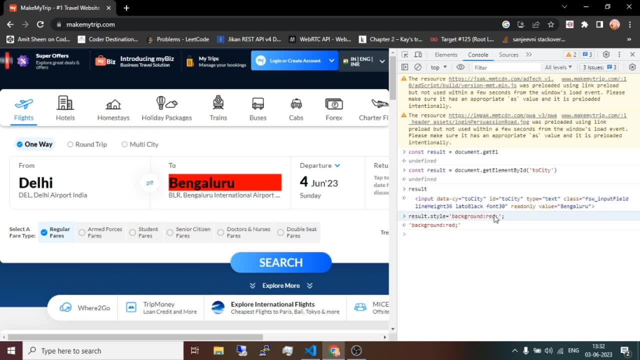 seeing I perform some, attach some style here. and the background of this input input field code automatically converted to red. so document dot get element by ID is a selector using which you can select any particular unique element from overall document. so let us move forward to the other selector in JavaScript. so let us move toward the 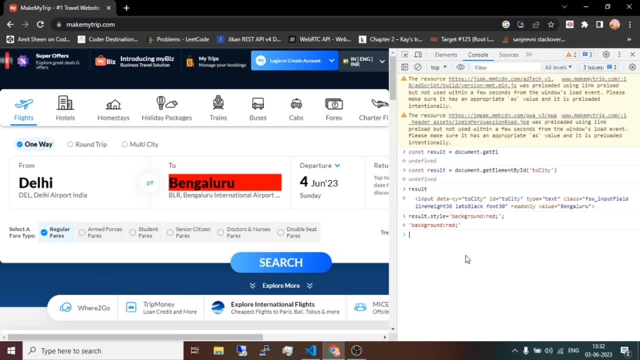 dot get element by class name. so, as I have explained earlier, the ID which is attached to any element inside the document is unique to that element, but in case of class, you can attach any particular class to any different kind of a number of element inside your website. it will return you all the element which are having that. 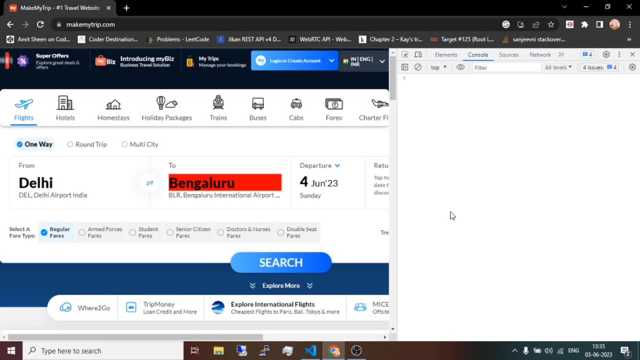 particular class and they in case of class, you can attach that any any particular class to any number of element inside the document. move forward the execution part of the selector. so I know what I am going to do. I am going to give a ticket燃3000 key of 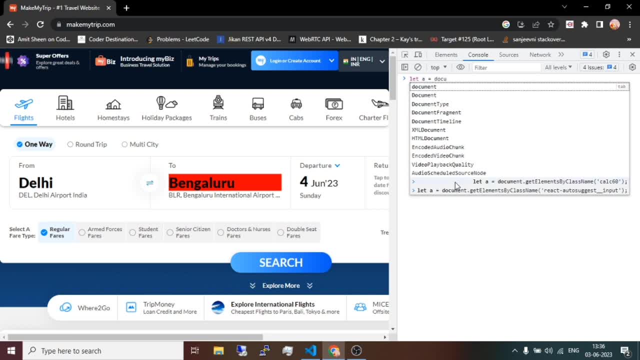 value. now I am going to create an item in class because we are going to have to activate the cleaningiguid too this time. so I am going to download in the bugs calendar. so I selected this class and let me see this layer. I can actually place it. 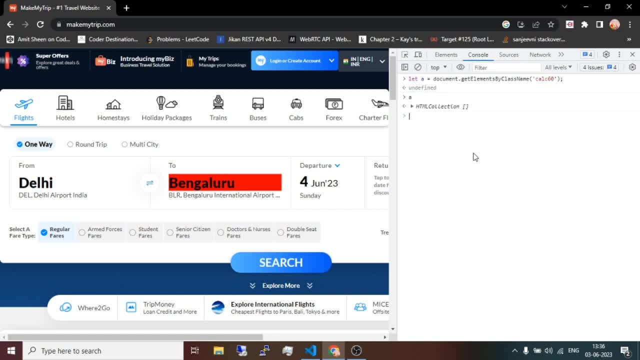 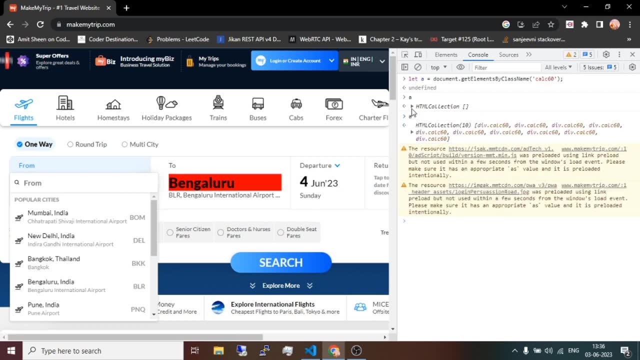 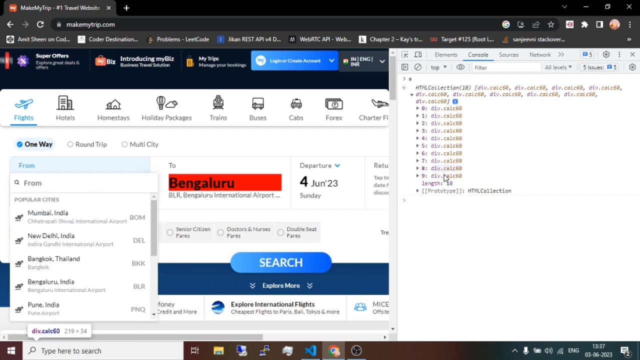 inside and then open a precipitation system. let me do all the things that it needs to create today. so now, here we are, getting the HTML collection of the different, this number of a cloud div element we are which are having this particular class attached to it. so by using document dot get element class name, you can access any number of 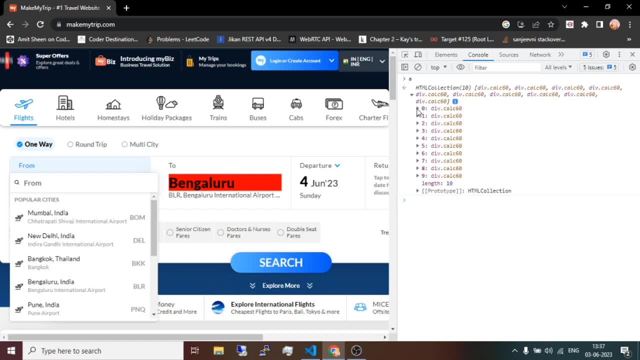 element inside the document which are having the same class and you can perform different kind of operation as per your logic on those particular class, says on those particular element inside the document. so let me perform some changes inside those particular div element in here. so first let me convert. 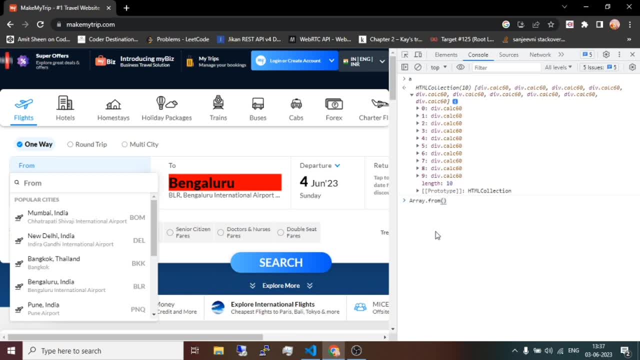 this HTML collection into a result, because inside HTML collection we didn't have any element inside it. so let me convert this HTML collection into a. so because inside HTML collection we didn't have any element inside it, so didn't get for each element, so I want to iterate over all the element added in a. 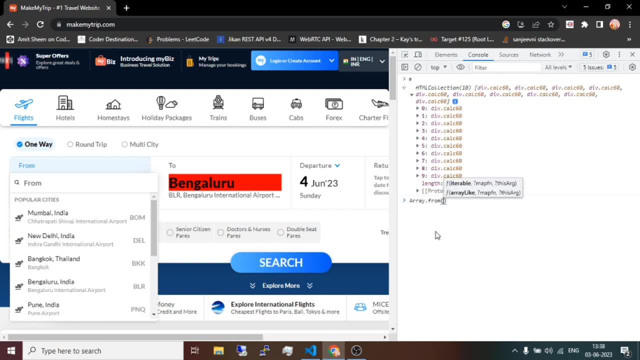 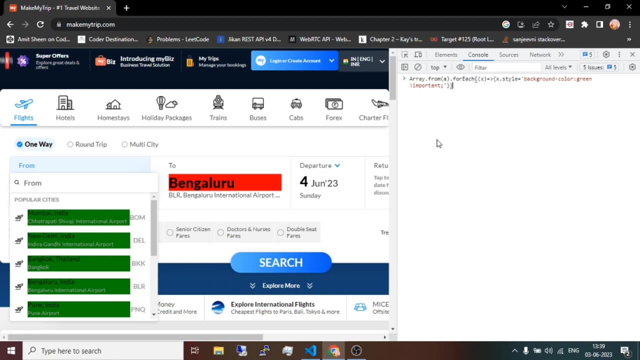 particular time, so let me convert it here and implement for each here. so here, in this method, I converted the background of all this element to green so, as we are seeing, the changes are also reflected here. so by using the document of get element by class, name you. 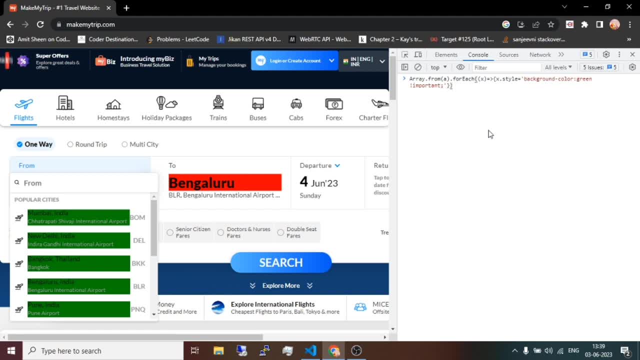 can access and a different kind of all number of element which are having the same class inside the document and perform some task for changes on that particular element. so now let us move forward with another selector inside inside the JavaScript, which is document dot get element by tag name. so as per it, 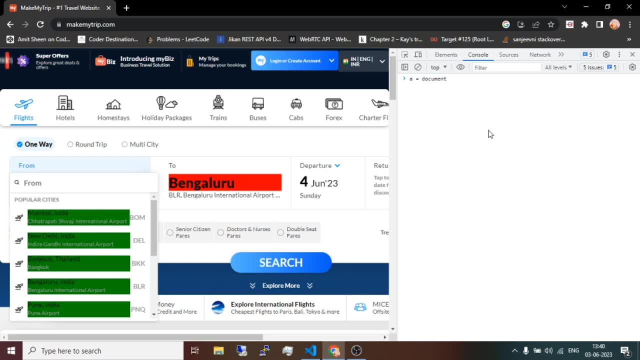 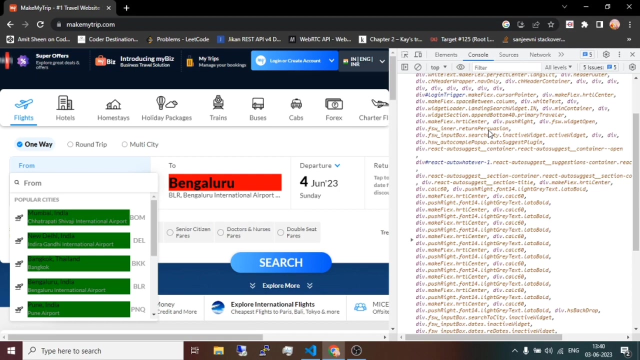 is clear by the definition of that method: get element by tag name. so. so by using this method we can get all the element of that particular tag name inside the document. so let me show you here. you, as you are seeing, we got all the list of div element in present inside this document as 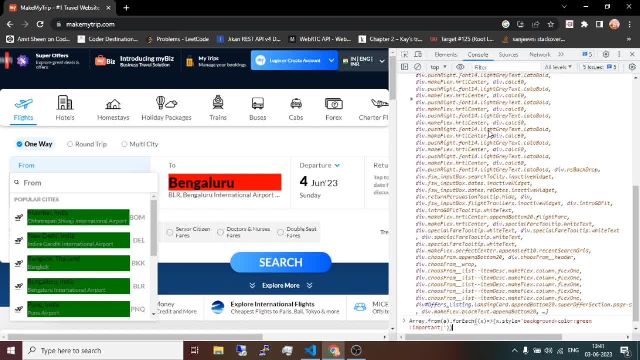 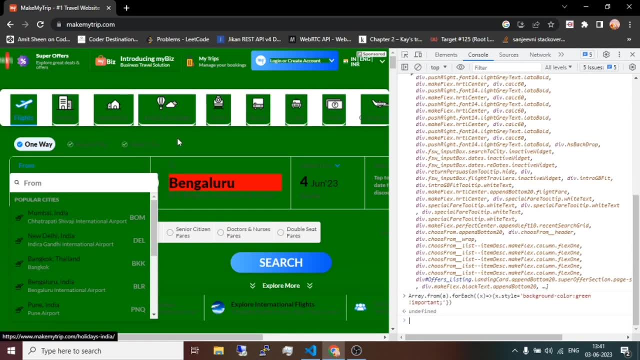 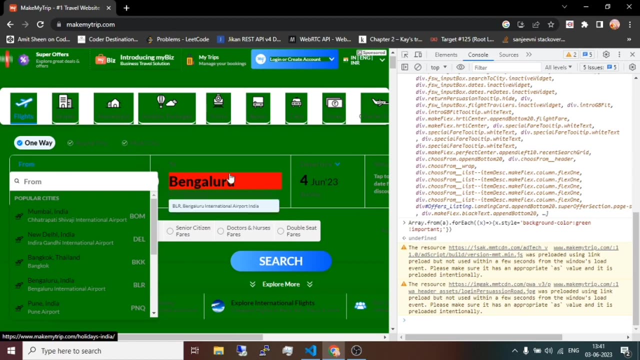 you are seeing here, so let me perform some task here as well. just copy pasting previous execution here: oh my god. so, as you are seeing, the background of all the div element which are present inside here got converted to green. it is eye-catching to me, but it is not good. 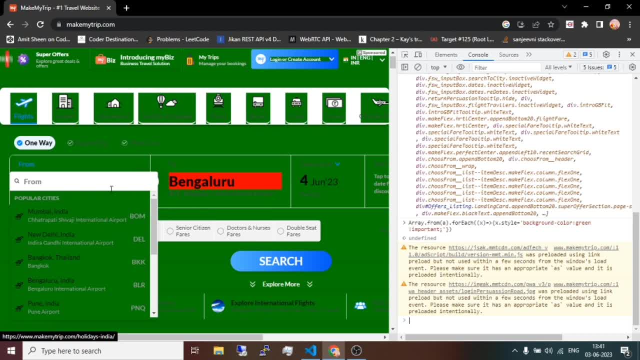 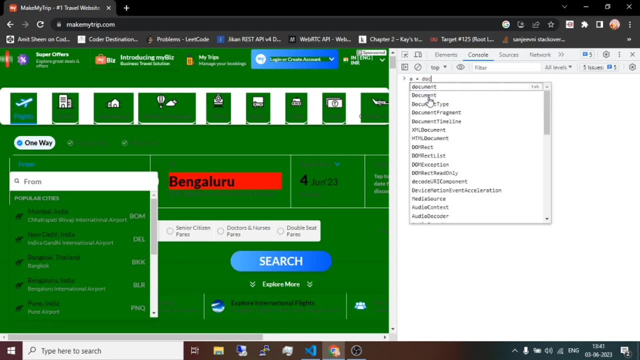 style, but I'm just saying it is looking good one way or another way. so let us move forward with the another selector inside the JavaScript, which is get element by tag name. so previously I explained get element by tag name, in which we can access any element using the tag name present in of that element. 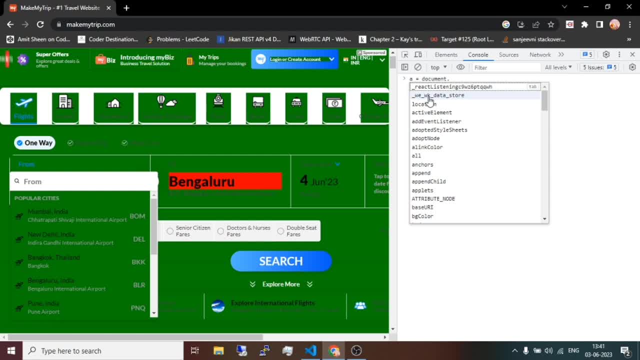 but in case of document dot, get element by name in this we will access. we can access any particular element using the name, whichever is assigned to that element. so I might not be able to find any element inside this website having particular name, so let us. I'm skipping that part here, but you can. 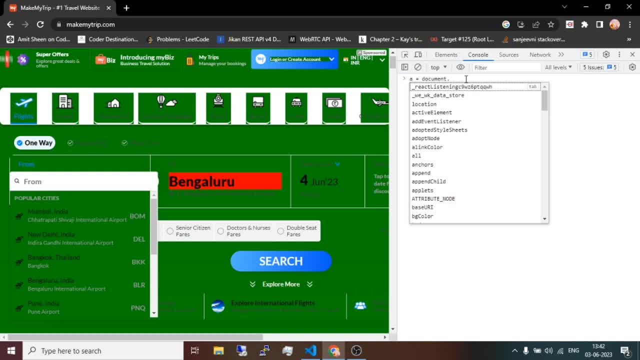 practice this JavaScript selector by yourself as well. now I'm moving forward with the query selector. so what does query selector will do? it will return you only one element at a time which is matching the criteria, whatever you provided inside the query here, so like if you are getting the hundred of element having the same class. 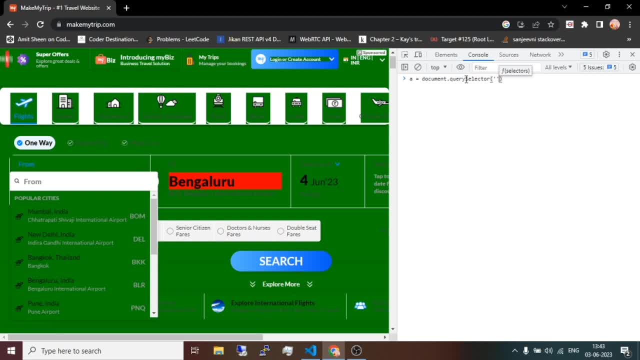 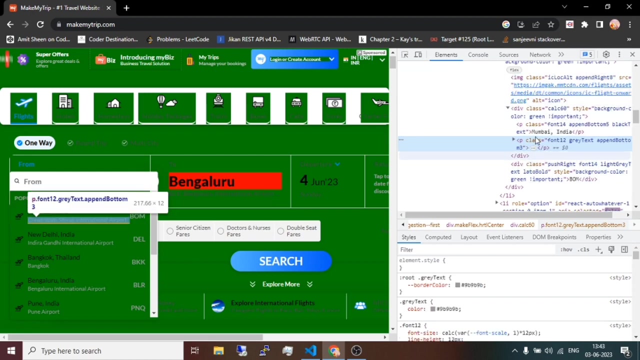 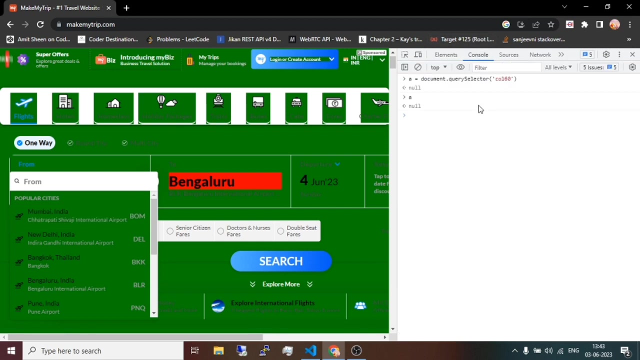 name, but it will only provide you first element which it encountered while traversing your HTML document. let me show you here. okay, I think I forgot something. let me check what was the class name? okay, the class name of cal sixty. so let me show you what we got. still no hope. okay, I forgot very important point. 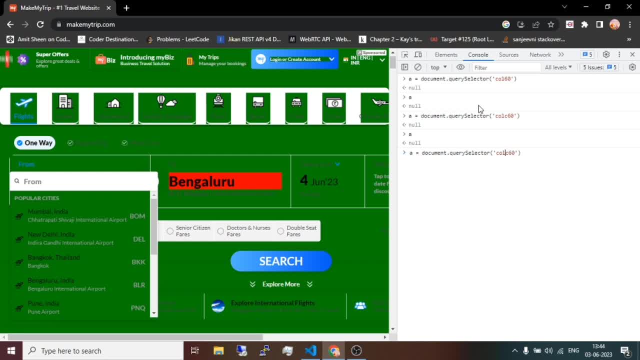 here. friends, let me explain you what I forgot here. so previously. in case of document dot get element by ID, by class name, by tag name, you just need to pass name of that particular tag, name of class or name of ID. you don't need to attach any prefix to it. but in 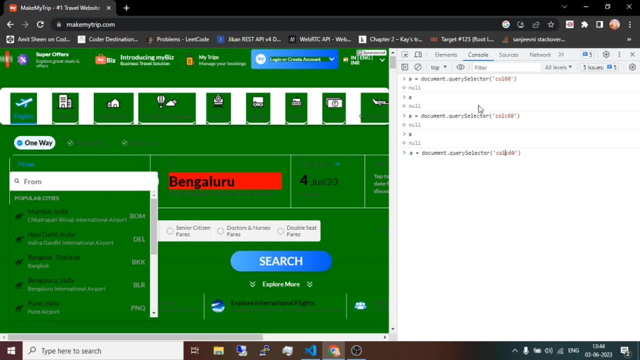 case of query selector, you need to attach prefix to it as well if it is a class. so if you are accessing classes like CSS, you attach dot to it and if you are accessing ID, you attach a pound sign in in prefix to that particular ID name. so, same as in query selector, you need to attach dot if you are accessing class here. 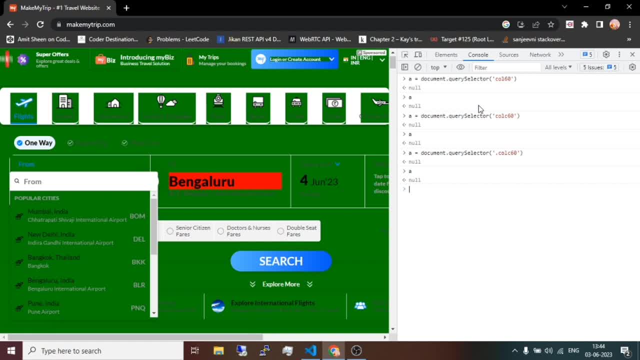 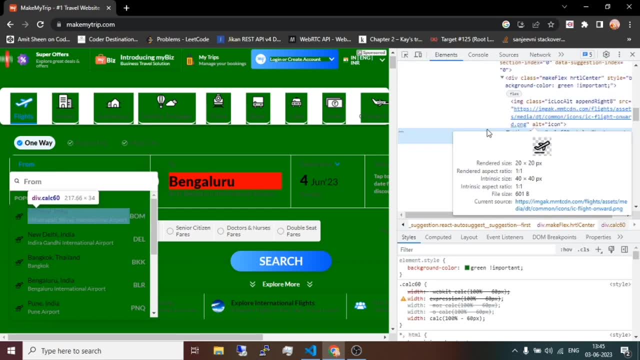 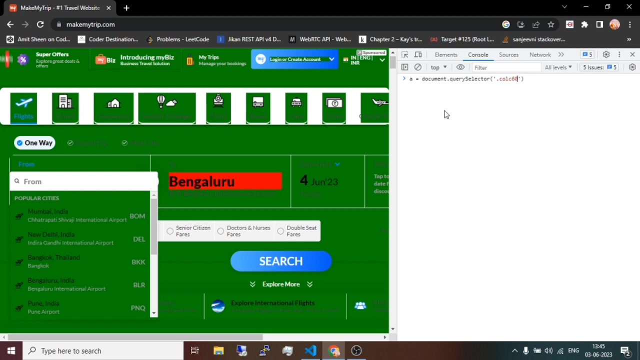 and so in other dumplings I used that paragraph. so the defense says that use variables code for employee means entity can use one, and one of them should be going to the following one, the. so let me show you here, let me show you here. so let me show you here. 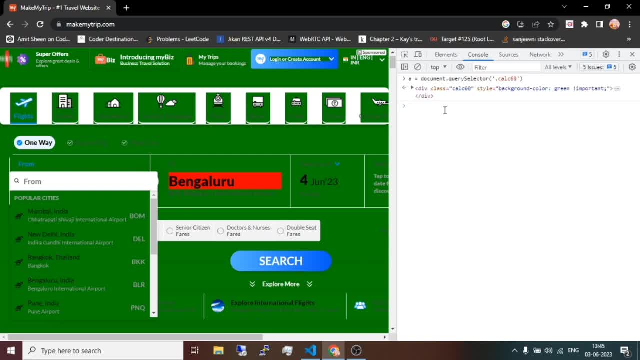 absolutely. let me show you here: finally, finally, finally, but gain, finally. Okay, we now get that particular element which we want to access here. So this calc60 is in between divs, So this class which we are accessing is attached to all the divs which are present in this. 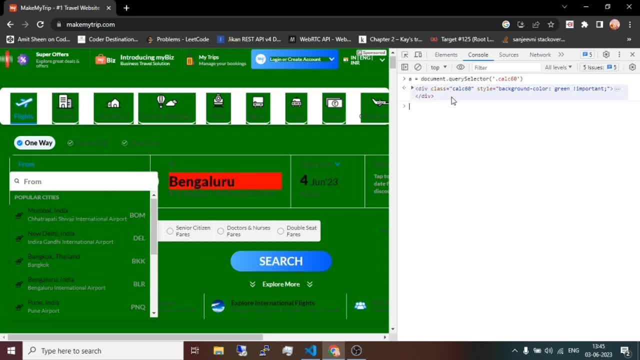 particular drop down here. So, but here we are only getting the first query selector. we only return one element at a time which is matching the criteria, whichever element it encountered, firstly in the traverse of the document. So let me make some style changes here. 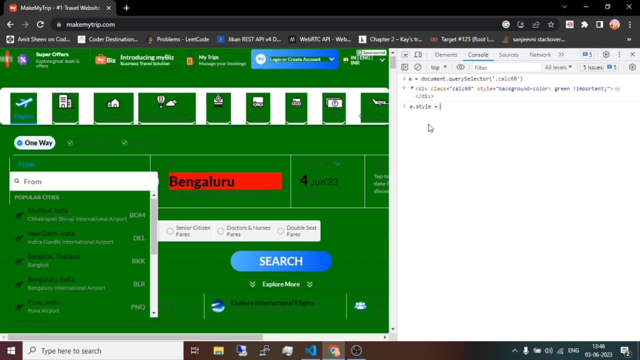 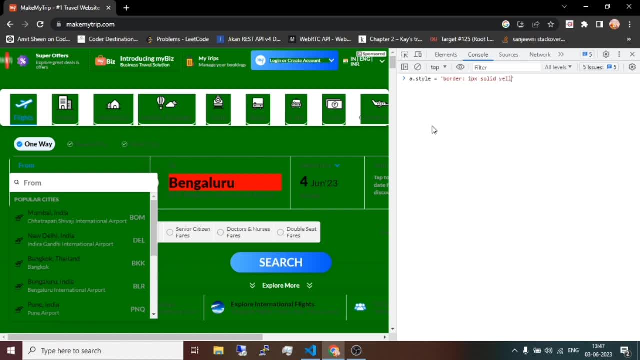 You might be thinking I am overly obsessed with the style of the document, maybe, so here I attached the border to this particular element here, which is one pixels solid yellow. so let us now move forward with the document dot query selector. all so you might be getting a little bit idea just by the name of this. 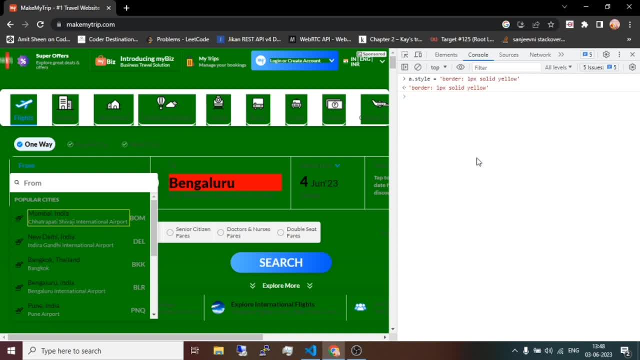 method. but in case just let me explain it to you. so the document dot query selector all method will return all the element which is matching the pass criteria in the query here. so, as I showed you previously, I was passing the class here and you got a list of number of drop-downs, so let me apply. 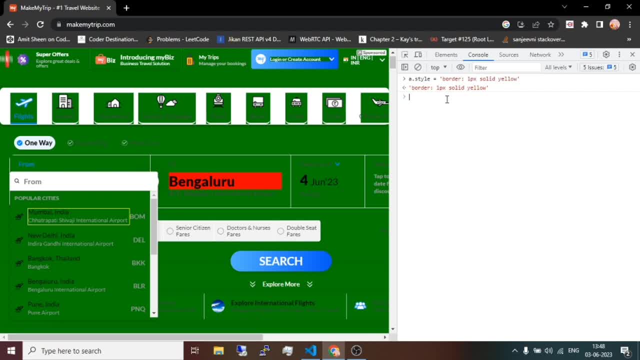 this document. dot query selector on this. these elements, so what so what? here we are getting the node list, the only pr element which are having this particular plus, etc. so all the div element which are having this particular element. you should notice that, byidi, we've 달라 plane in this. 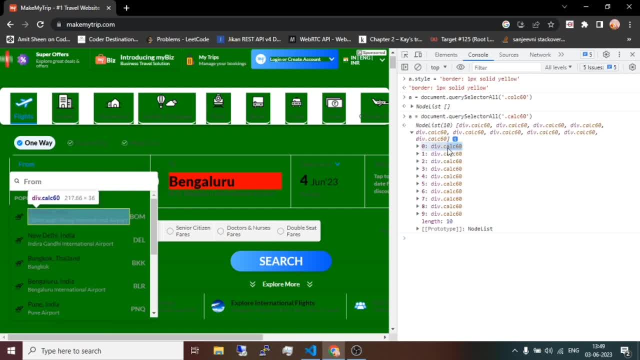 particular stop À scope, particular class attached to it. we are getting all the developments here in the form of node list, so same, as i previously said, in the class name you can perform change style of this, all the particular development here. so this is it for the video. so if you like the video, please subscribe. 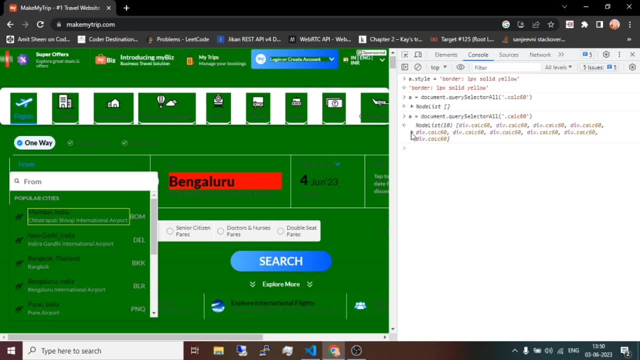 the channel. it's a small request from you as a uh. please subscribe the video and please press the bell icon so you can get notified whenever i upload new video to my youtube channel and also share this video to your friend if you find this video helpful to you. so 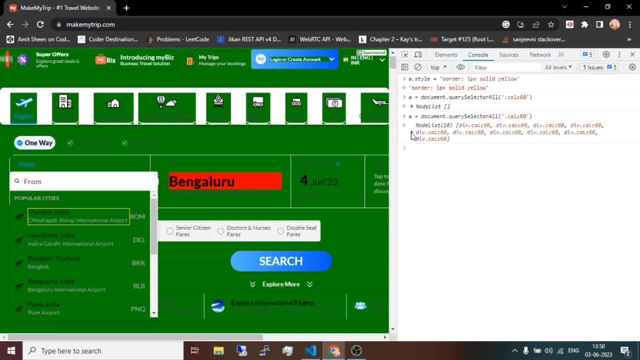 they can also learn these amazing concepts. so thank you, friends. we'll meet in next video. bye.